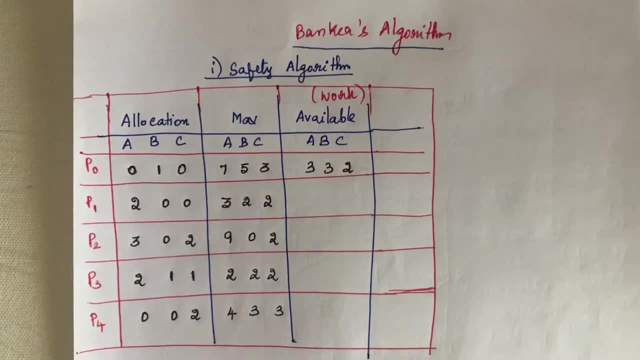 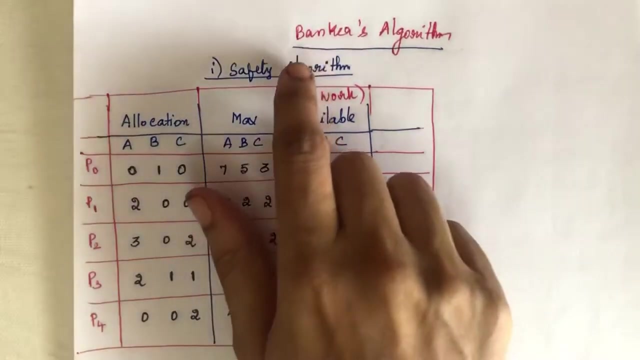 algorithm also, we can avoid deadlock. so if the resource type is single, if you have only one single instance of resource type, then we can use resource allocation grab scheme. but if the resource contents contain many types, then we should use Banker's algorithm to avoid the deadlock. So if the resource instances is multiple, then we should use Banker's. 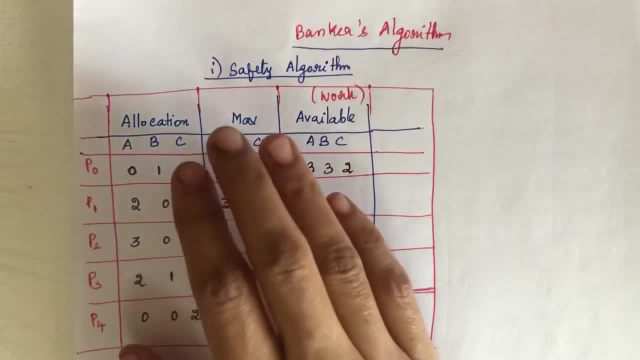 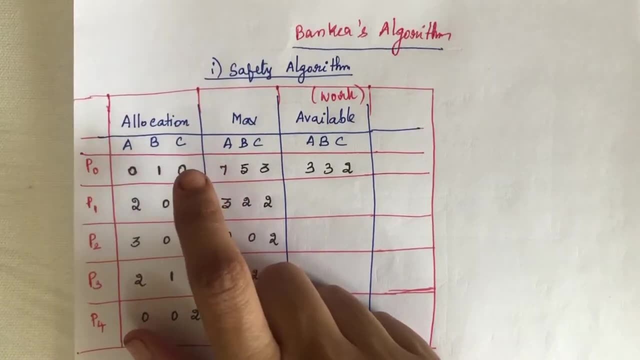 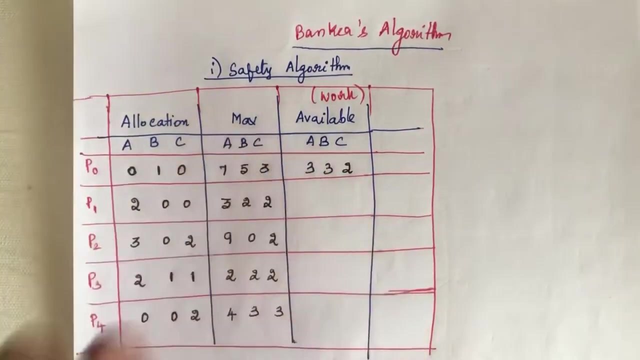 algorithm to avoid the deadlock. that is what we are going to see now. So in bankers algorithm we can do this bankers algorithm in two ways again, the first is safety algorithm. the second one is request resource request algorithm. that we will see it later. first come into safety algorithm. okay, so why this name is called as bankers algorithm? because the name. 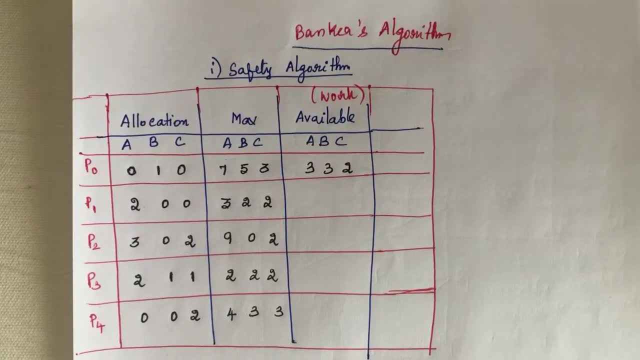 was chosen because algorithm can be used in any banking system. it will ensure that bank never allocate the cash to any one of the person if it could not able to satisfy the need of all the customers. so the bank will check, will ensure that if the bank can able to satisfy the need of all, 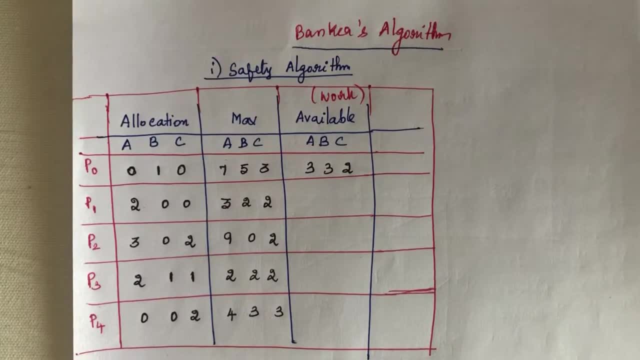 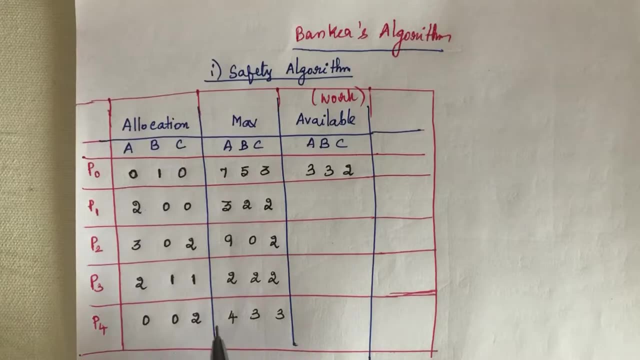 the customers, then only it will allocate the cash to the persons, or otherwise it will not allocate. that is why it is called safety algorithm. so the main criteria for bankers algorithm is so: whenever any process enters a system, it must declare the maximum number of resources it requires to complete its execution. and this 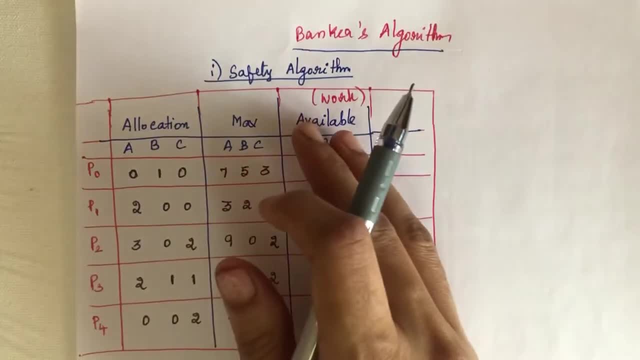 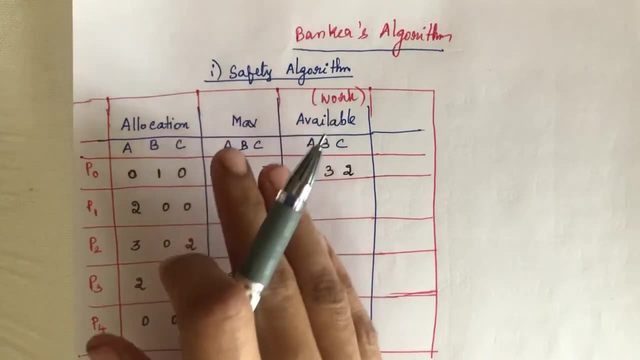 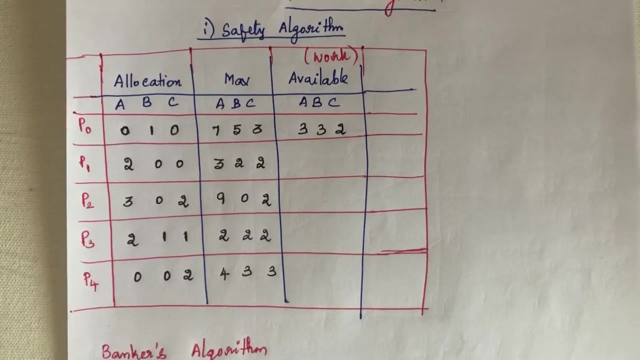 number should not exceed the total number of resources in the system. okay, so let's move on to the safety algorithm. using this algorithm, you will find whether or not system is in safe state. okay, that is what we are going to determine using this safety algorithm. so here we they have given. 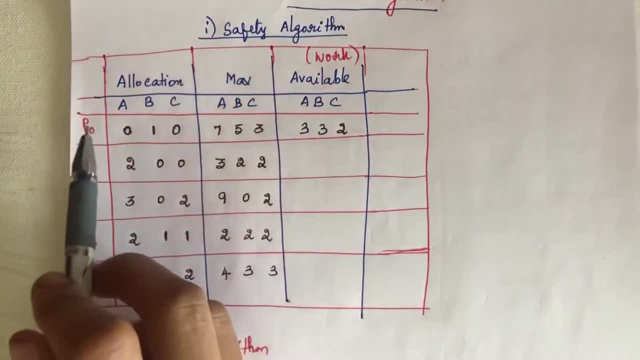 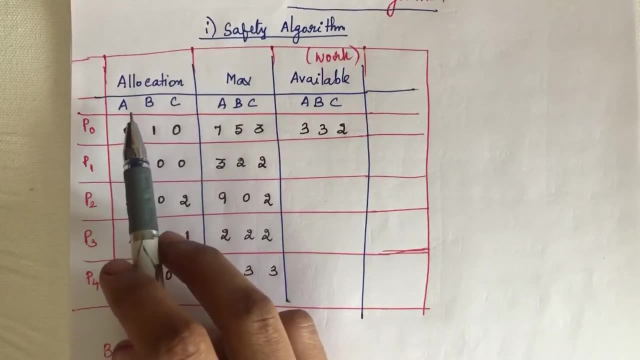 you the allocation, then maximum and available. so there are five processes naming, from p0, p1, p2, p3 and p4 and there are three instances, that is like three resource type. one is a, b and c. so resource type may be printer. so printer is named as a scanner can be named as b or otherwise some other. 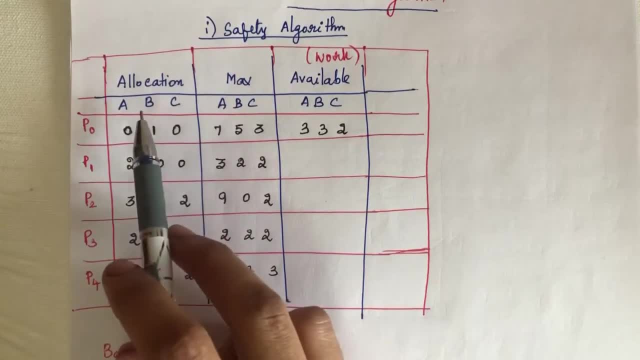 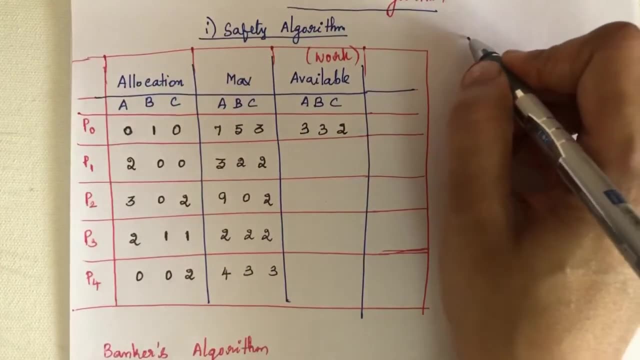 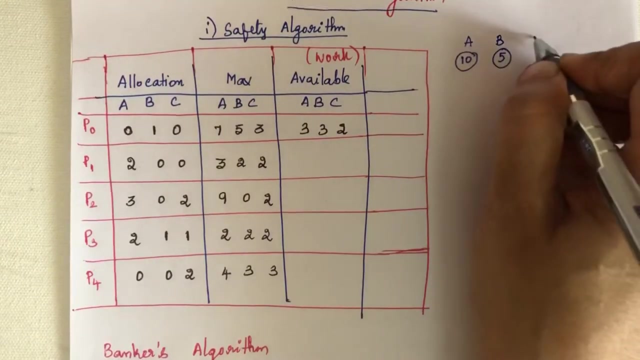 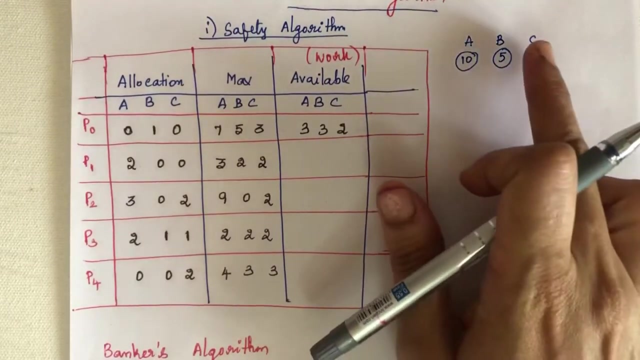 ram can be named as c. likewise any resource type will be there. so there are three resource type attached to the system, So a, b and c. so here in the system a is having 10- 10 instances of a and b is having five instances and c is having seven instances. initially a is having 10 instances and b is having five instances. 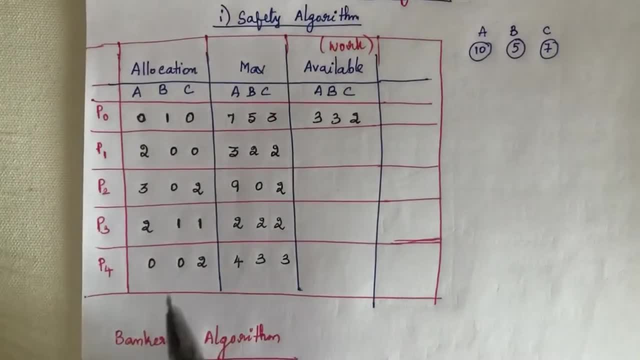 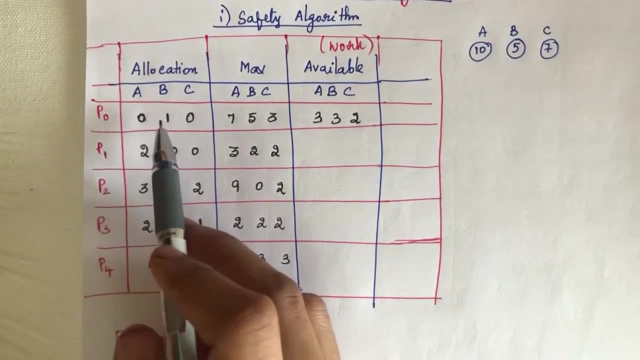 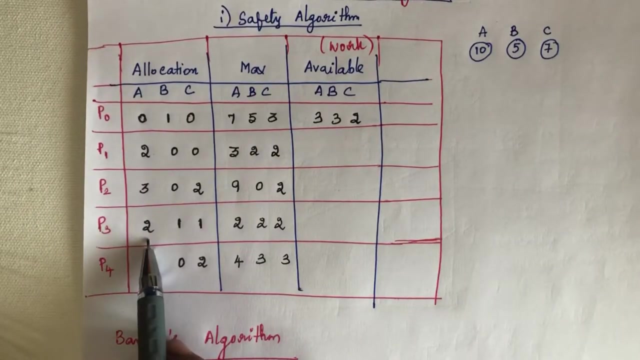 and seven is c is having seven instances. okay, so we will see this. so in this out of 10, so this a, so out of 10, the system is allocated two instances for p1, three instances for p2 and two instances for p3. so totally it is. 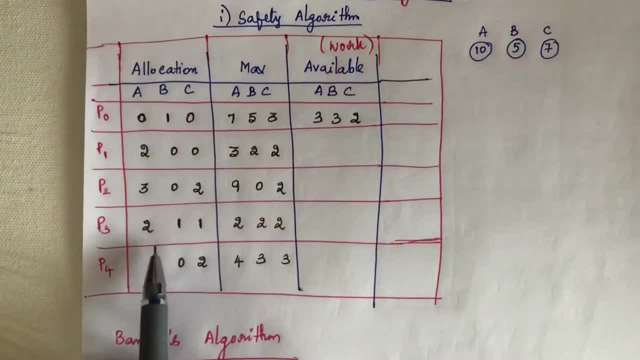 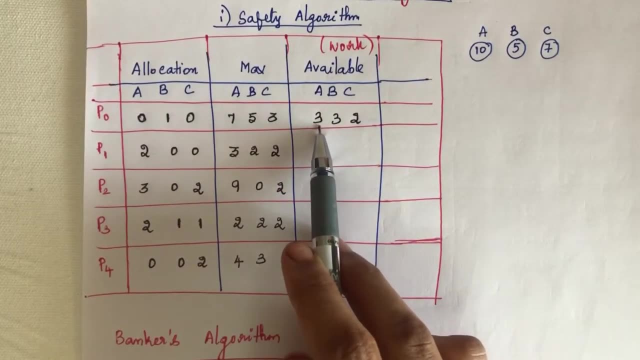 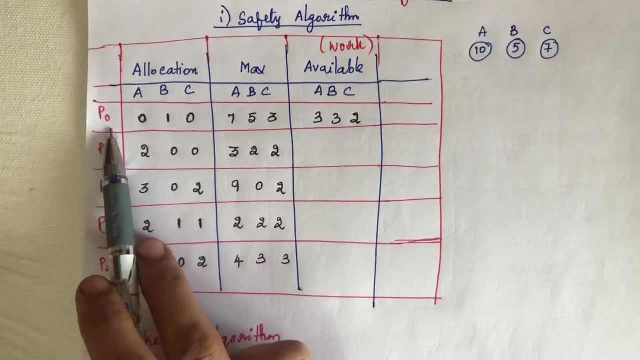 three, four, five, six, seven. so out of 10, seven has been allocated. so available resources in the system is three. that is what i have written here. available resources in the system is three out of five instances of b type. so how much it is allocated. so one has been allocated to p0 and one is allocated. 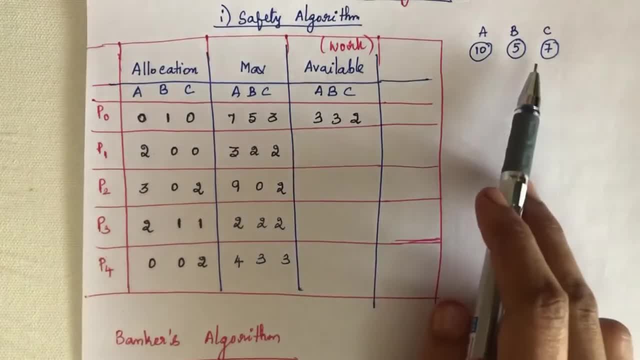 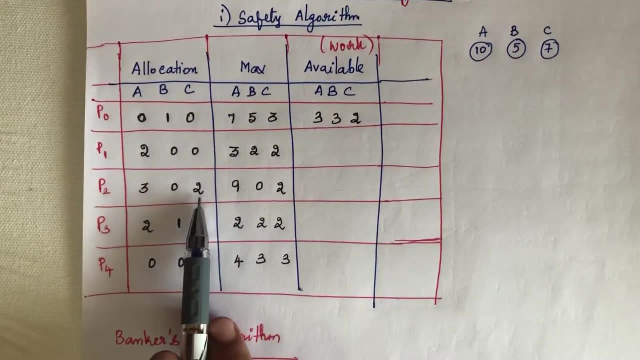 to c. now let us see how many instances have been allocated. remaining three is available in the system. Next come into c: c out of seven. so seven instances, so out of seven. so the system has allocated two instances to p2 and one instance to p3 and two to p4. so it is two, one, two. that is nothing but five. 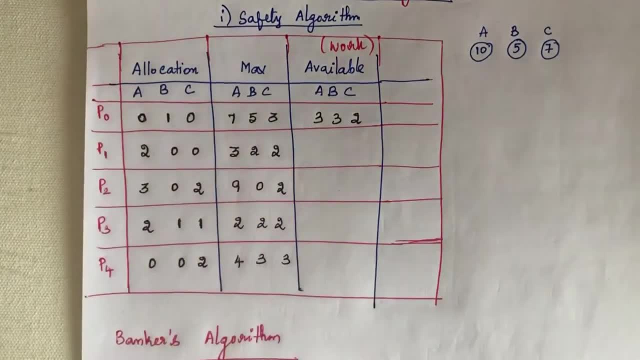 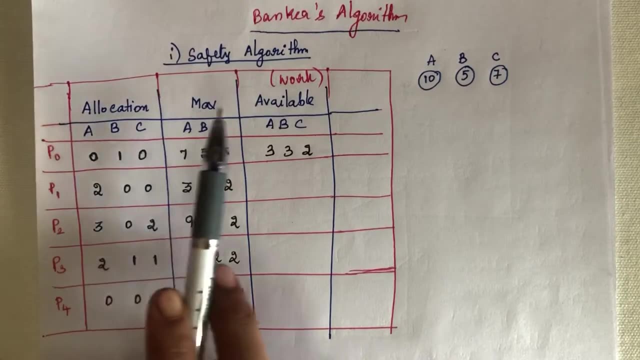 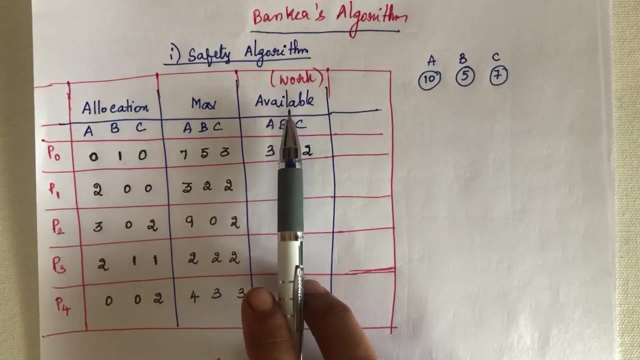 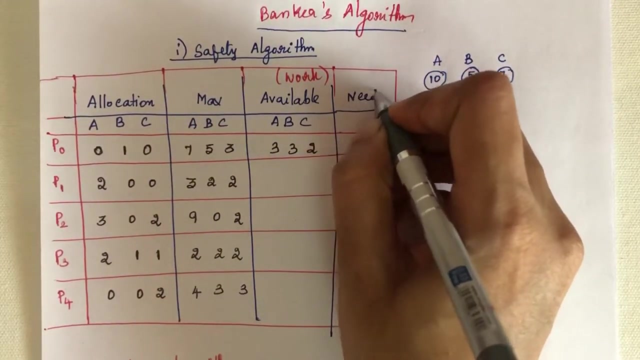 so seven minus five it is two, so two are remaining here. so in this allocation it specifies the resources current allocated to each process and maximum specifies the maximum demand of each process. okay and available is available resources in the system. so first we need to determine need, need, matrix. 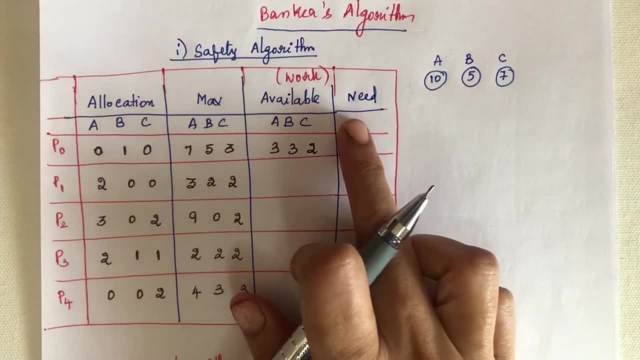 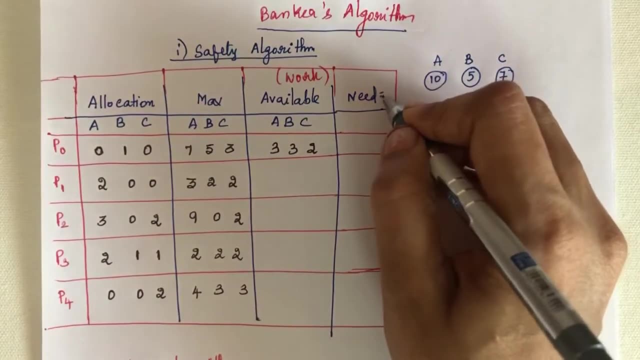 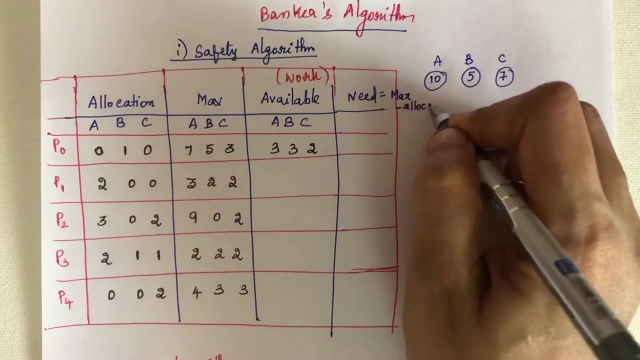 what do you mean by need matrix? so this value specifies the additional resources that process may still require to complete its task. so the need matrix can be calculated with the formula of max minus allocation. so when you use this formula you will get a need matrix of each process. 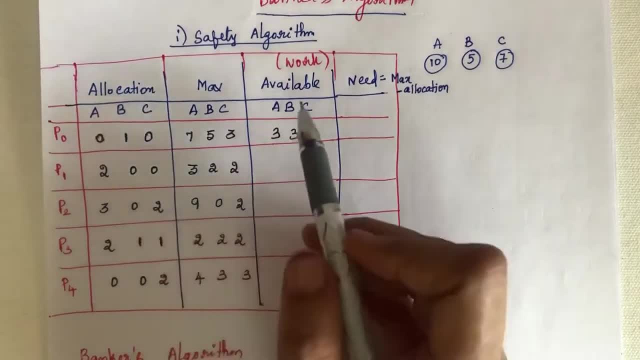 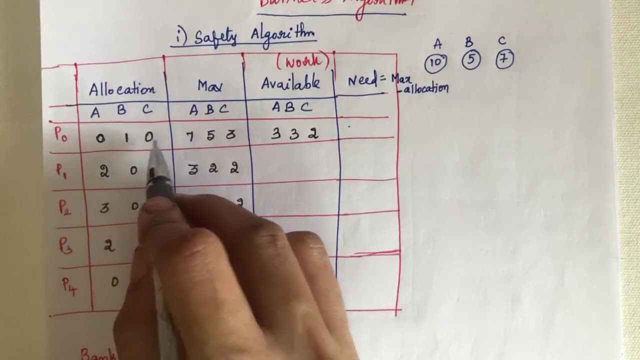 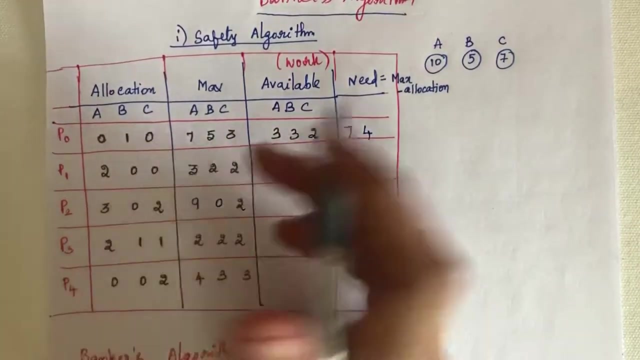 so it is maximum minus allocation. so what is need for the process? p naught, it will be 7, here it is 0, 1, 0, here it is 7, 5, 3. so 7 minus 0 is 7, 5 minus 1 is 4 and 3 minus 0 is 3, and for: 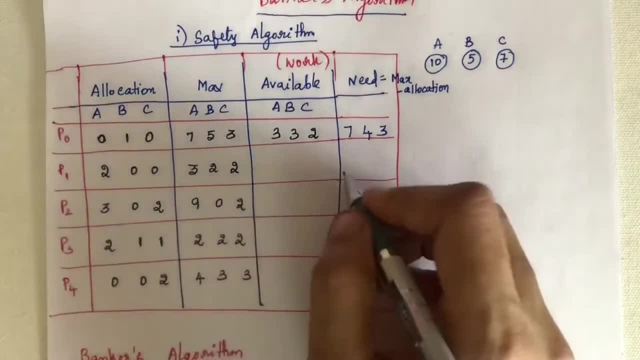 the process p2. the need matrix is 7: 5- 3, so 7 minus 0 is 7, 5 minus 1 is 4 and 3 minus 0 is 3. Need matrix is: 3 minus 2 is 1,, 2 minus 0 is 2 and 2 minus 0 is 2.. 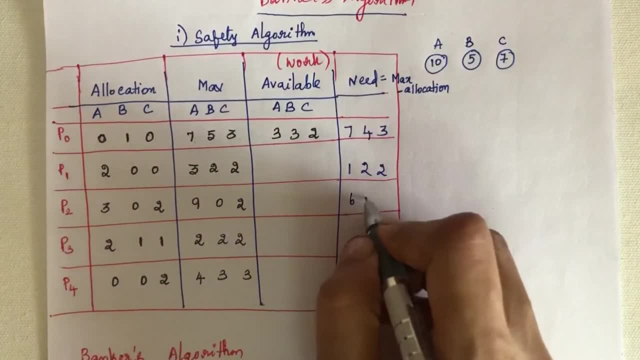 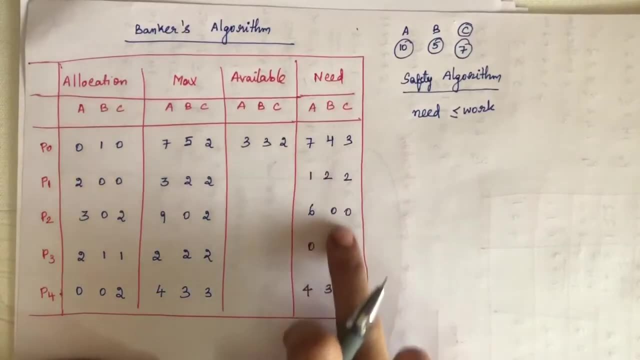 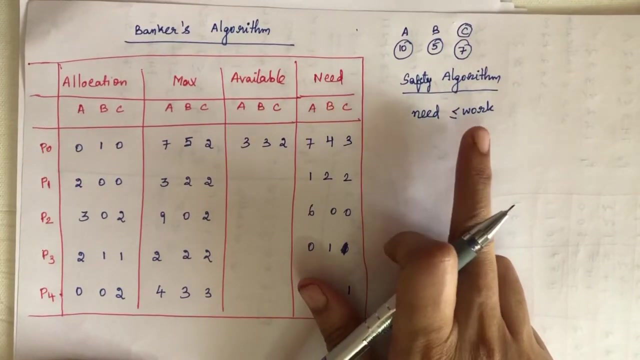 Like phase, we will calculate for other values also. it will be 6, 0, 0,, 0, 1, 1,, 4, 3, 1.. After finding the need value for the safety algorithm, the formula used is: need value should be lesser than or equal to work. 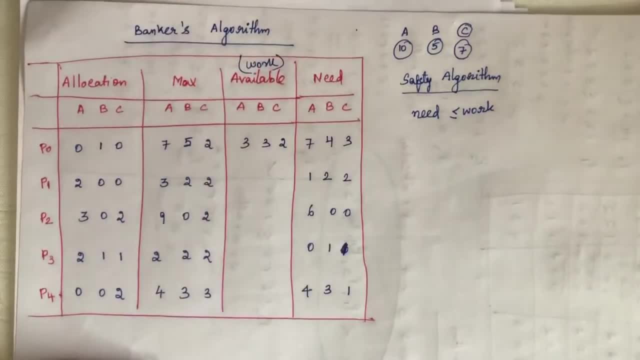 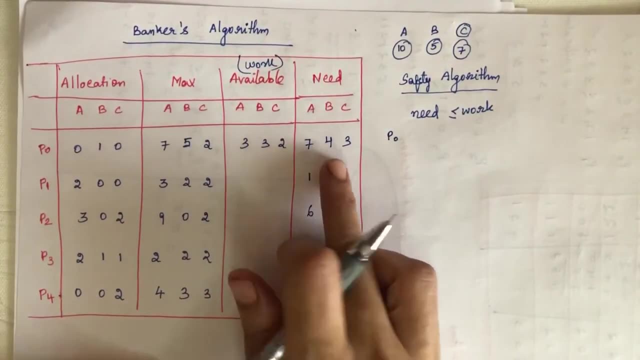 Work is nothing but available number of resources in the system. So first we will consider the process P0.. So for the process P0 the need value is 7 4 3.. 7 4 3 is lesser than or equal to the work 3 3- 2.. 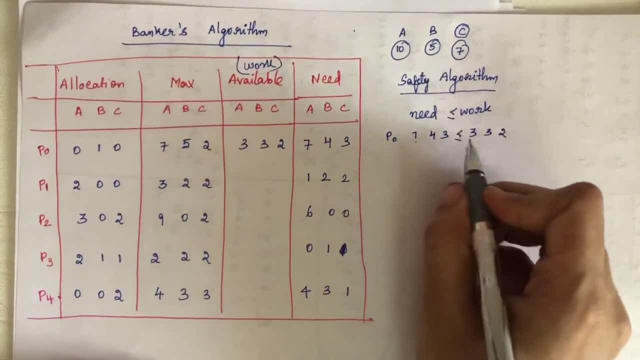 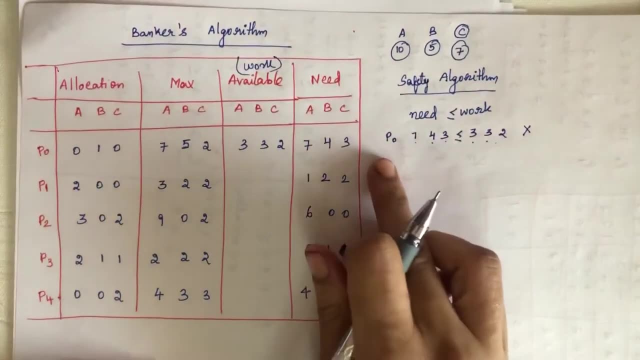 So it is 3, 3, 2.. We need to check: 7 is lesser than or equal to 3, 4 is lesser than or equal to 3 and 3 is lesser than or equal to 2.. No, So we cannot allocate the resources to the process P0 first. 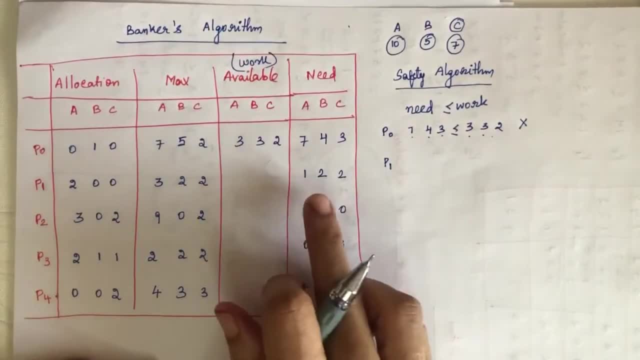 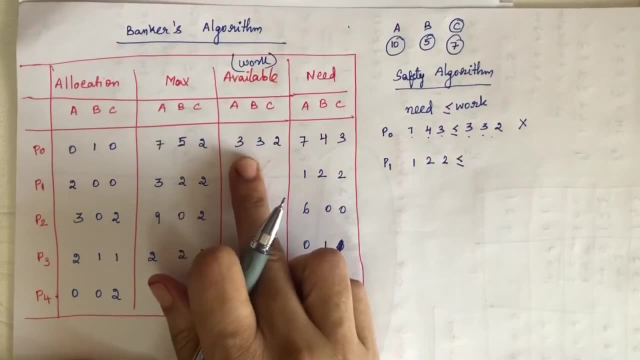 Next we will go for checking P1.. So for the P1, what is the need value? it is 1 2, 2.. So 1 2 2 is lesser than or equal to the available resources. that is, 3, 3, 2, 3, 3, 2.. 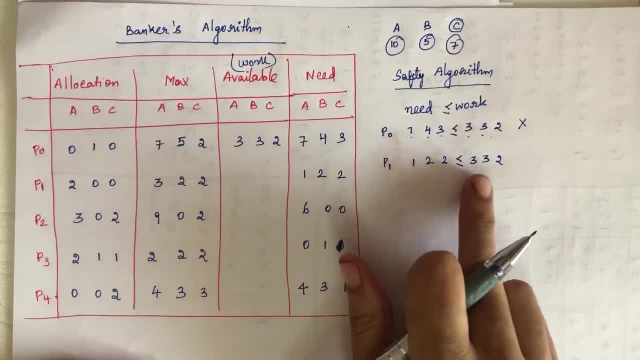 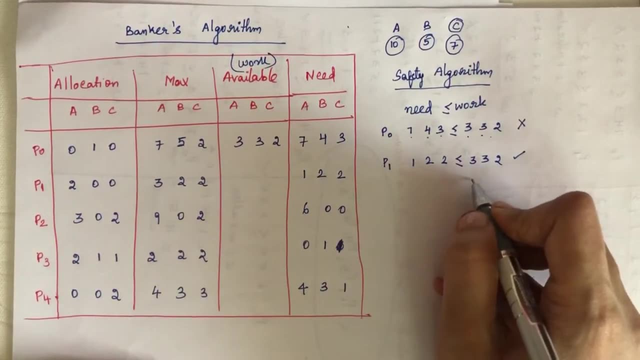 So here 1 is lesser than or equal to 3, 2 is lesser than or equal to 3, and 2 is lesser than or equal to 2.. So we can allocate resources to the process P1.. So what is the new work value? 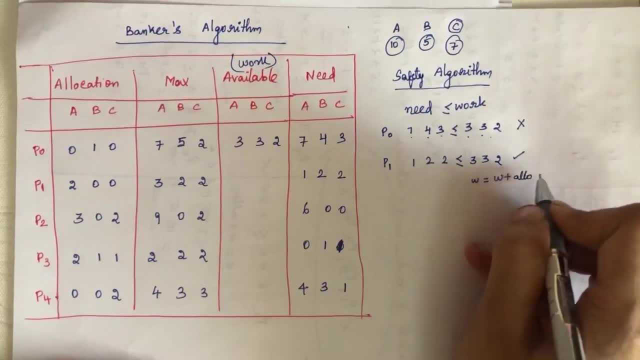 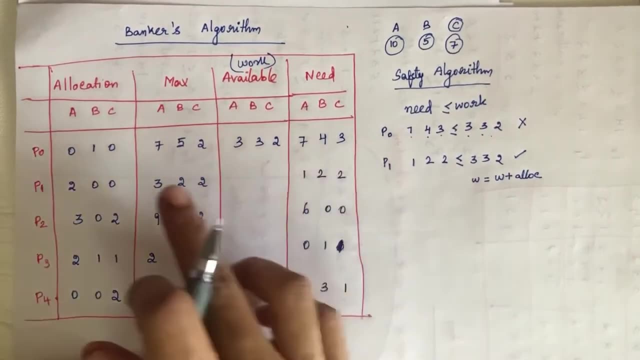 Work value will be work plus allocation, Work plus allocation. So allocating this resources to the system now, the process P1 will complete its execution and it will return back the resources to the system. So the new work value will be work value plus allocated value. 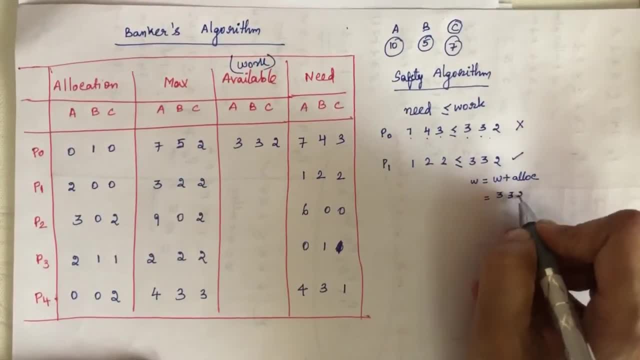 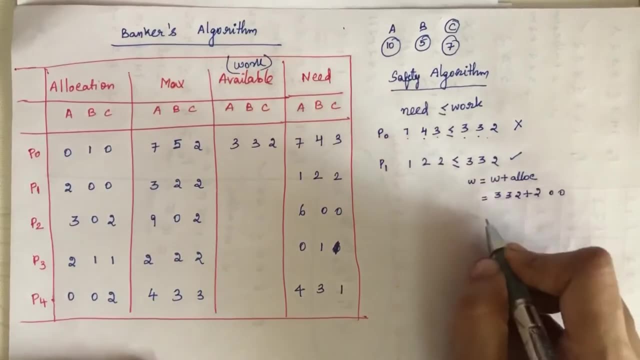 What is work value? Here it is 3, 3, 2 plus allocated value. What is allocated? How many resources have been allocated? 2 0 0, 2 0, 0.. So it will be 3 plus 2, 5, 3 plus 0 is 3 and 2 plus 0 is 2.. 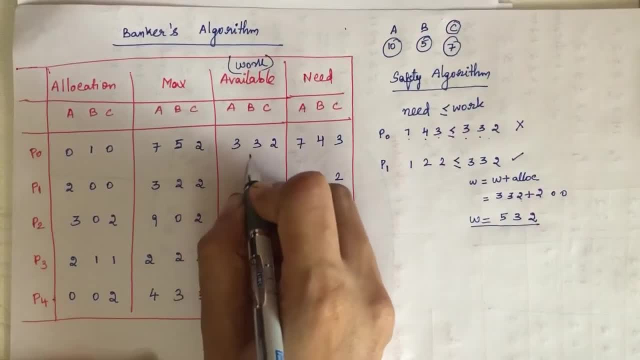 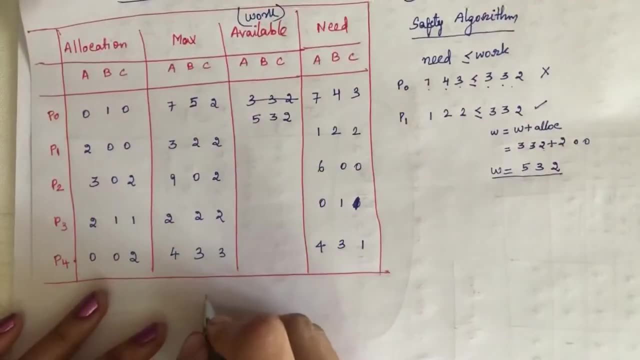 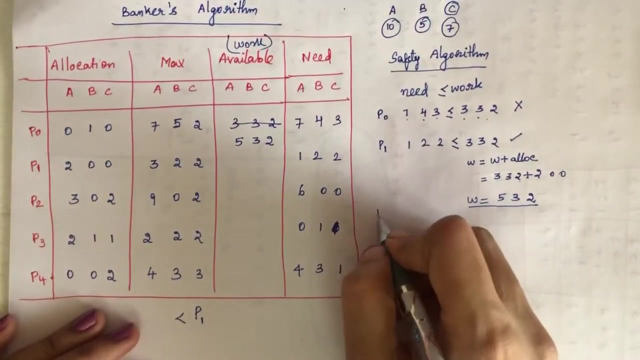 Okay, This is the new work value that we will change it here. it will be 5, 3, 2.. Next we will check for. so we will keep on safe state sequences. first we are allocating the resources to the process P1.. Now we will go for checking P2, P2 process. 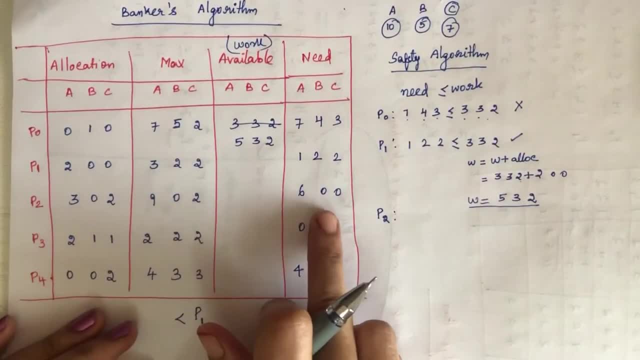 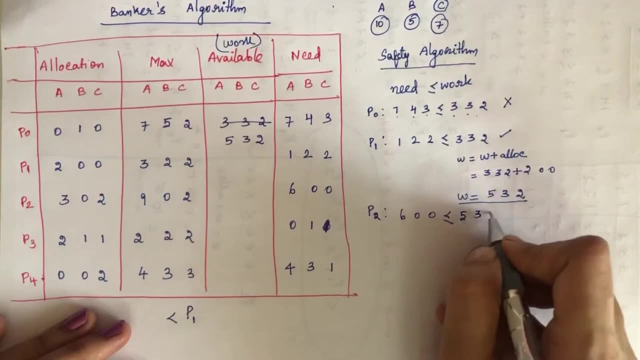 What is? what is the need value for the P2 process? it is 6 0 0.. So 6 0 0 is lesser than or equal to. the new work value is 5 3 2, 5 3 2.. 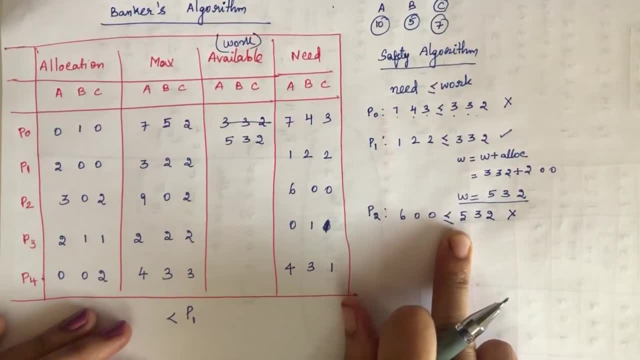 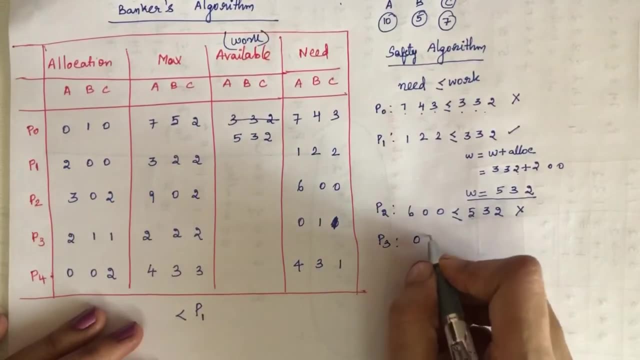 So here it is not lesser. 6 is not lesser than or equal to 5.. So we will not allocate the resources to P2.. Next we will go for checking P3,. P3, the need value is 0, 1, 1, which is lesser than or equal. 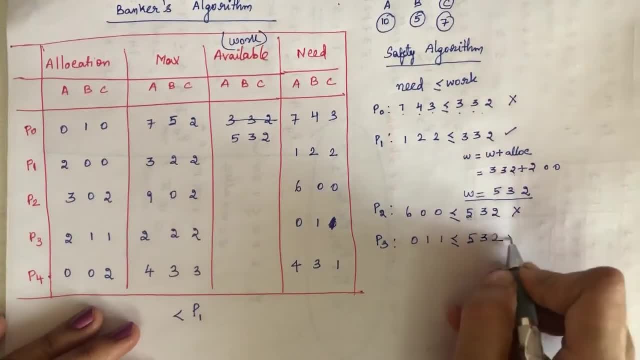 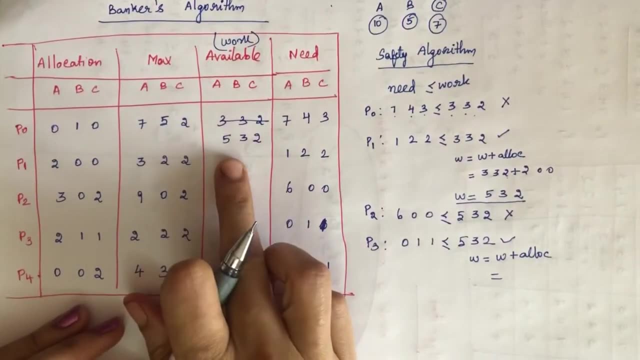 to the work value, that is 5, 3, 2.. So here it is lesser. So we will calculate the new work value. work value will be work plus allocation. What is the work value? it is 5, 3, 2,. 5, 3, 2 plus allocated value. for P3 is 2 double 1,. 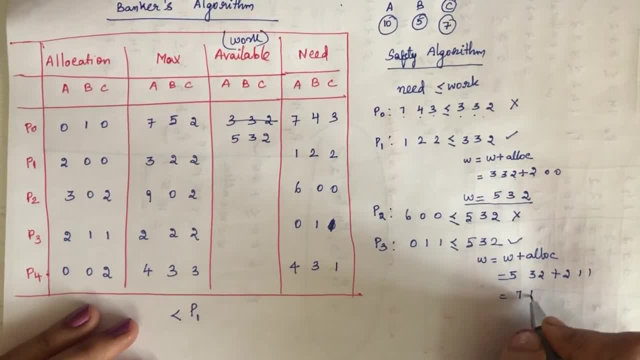 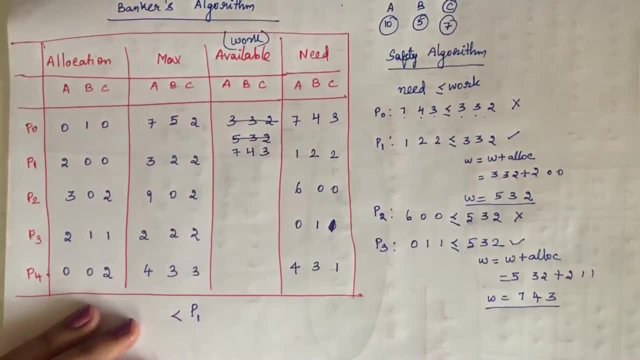 2 double 1.. So it will be 7, 3 plus 1 is 4, and 2 plus 1 is 3.. So this is the new work value. So we will change it in the system: 7, 4, 3.. 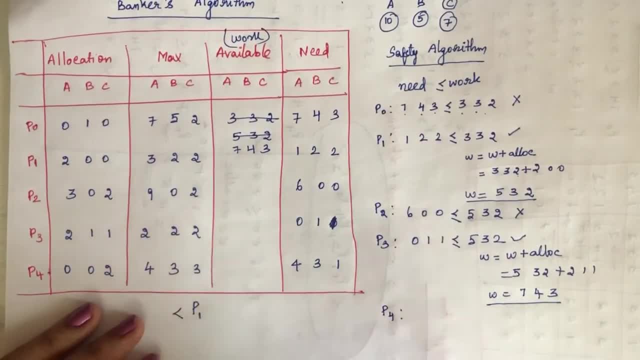 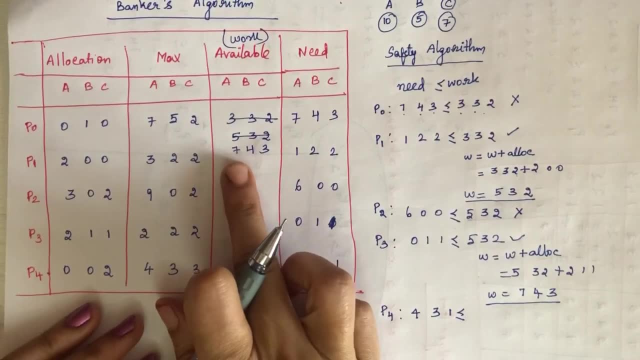 So now we will go for the process P4.. So what is process P4, what is the need value here? it is 4 3. 1 is lesser than or equal to the new work values 7 4 3, 7 4 3,. yes, it can be allocated right. 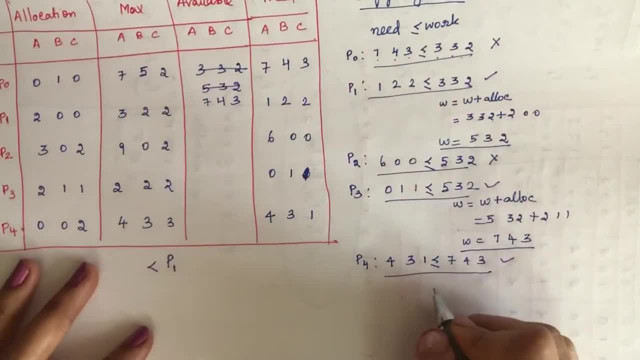 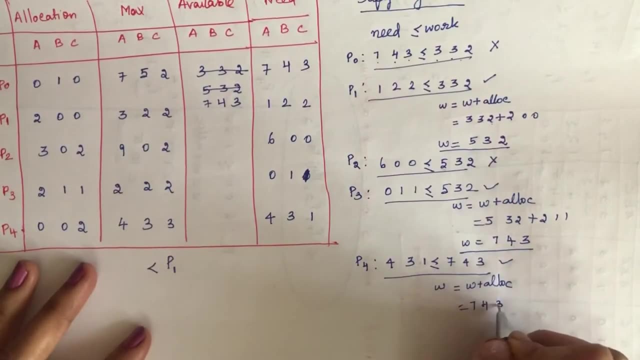 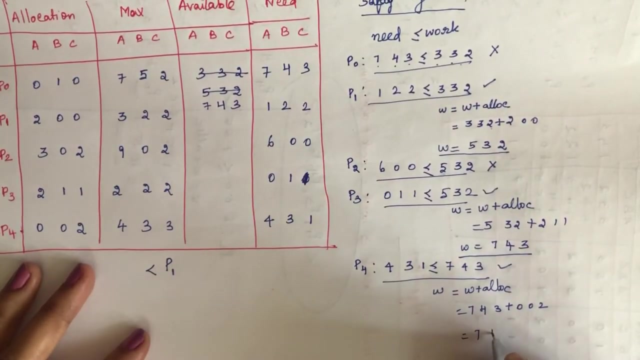 So it can be allocated. So we will find out The new work value. that will be work plus allocation work values: 7 4, 3, allocated values for the process P4. it is 0 0, 2,, 0 0, 2. it will be 7 4, 5. ok. 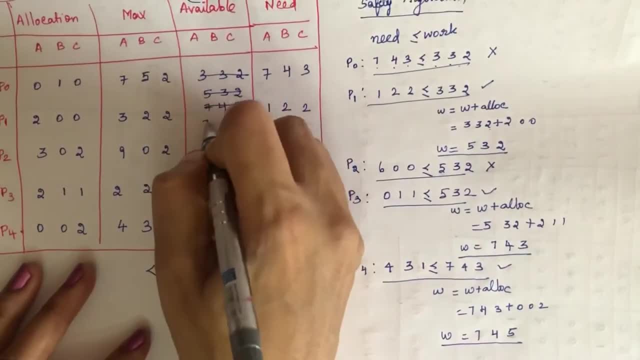 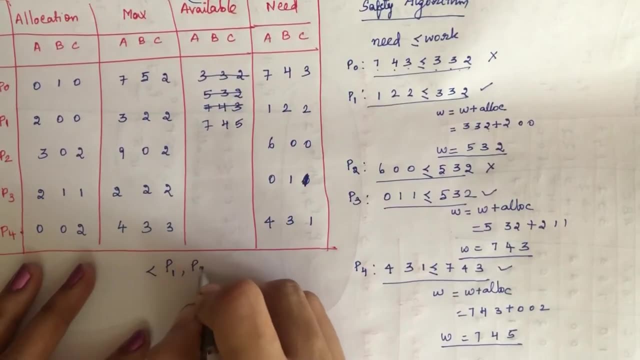 So this 7 4 5. we will change it in the available resources: 7 4 5.. So first P1 has entered the safe state and P3, P3 has entered, now P4 has entered. So we have completed one cycle. 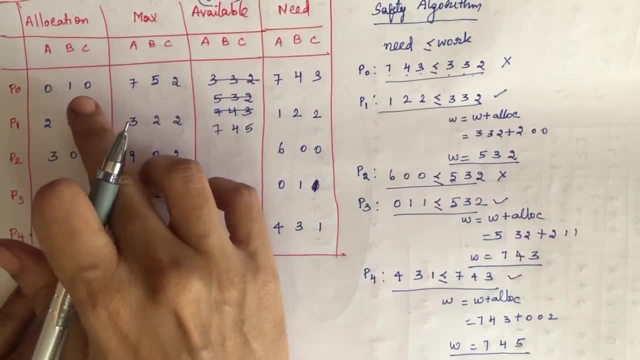 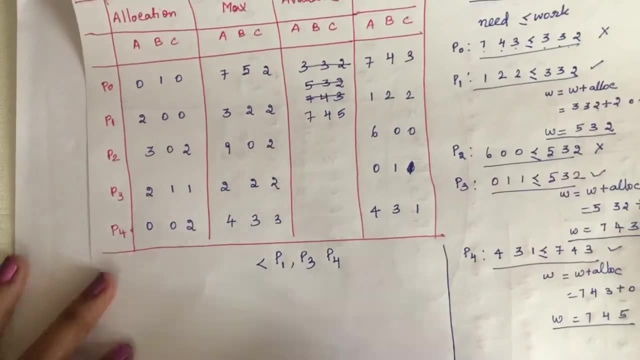 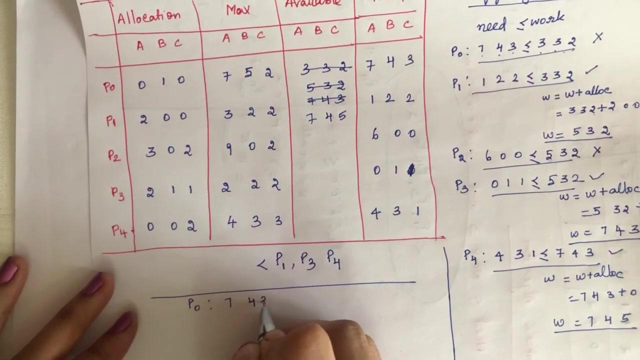 We will go for checking the next process which has not been allocated. So P0 has not been allocated. So again, we will check it for the process P0 now. So P0, what is the need value? here it is 7, 4. 3 is lesser than or equal to work values. 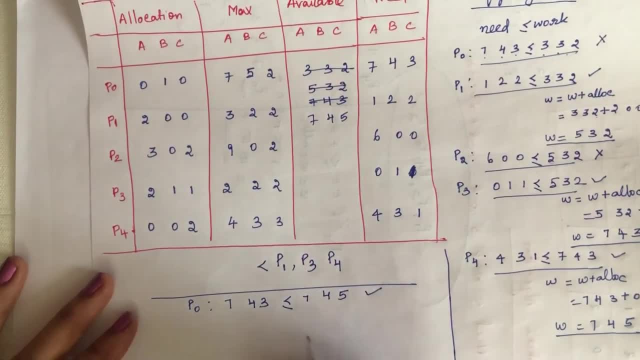 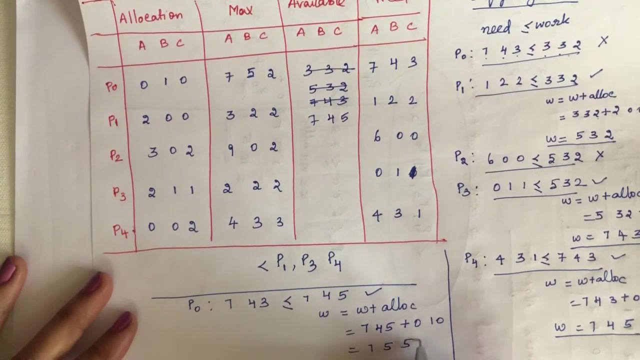 7, 4, 5,. yes, it is lesser, So we can allocate What is the work value. It will be work plus allocation Work value: 7 4, 3.. 6 4, 5 plus allocated value for P0 is 0 1, 0. it will be 7 5, 5. ok, that is the new work value. 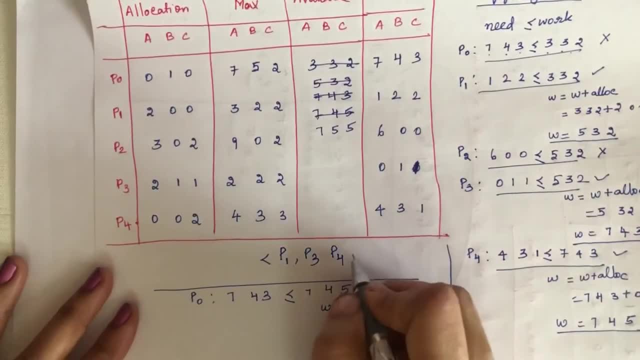 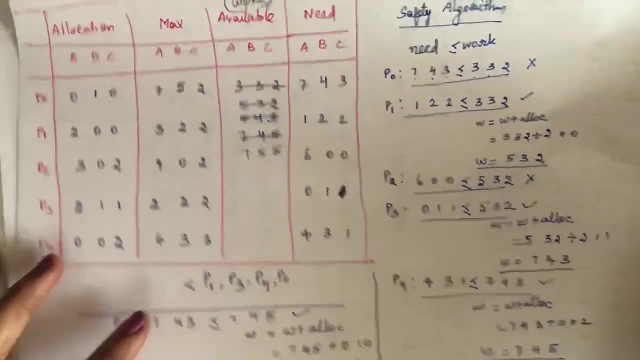 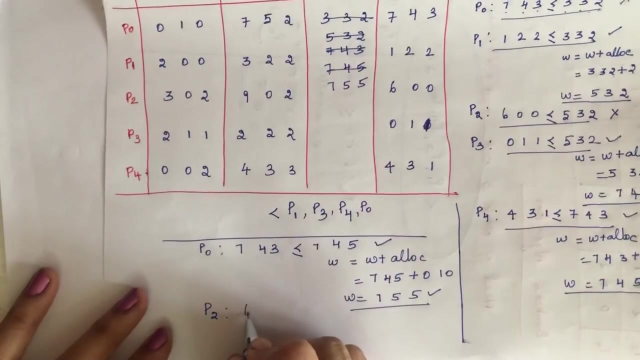 So it will be 7: 5, 5.. So this P0 also enters the safe state. Now we will check for. the next process which has not allocated is P2.. So the last process is P2.. So P2, the need value is 6 0, 0.. 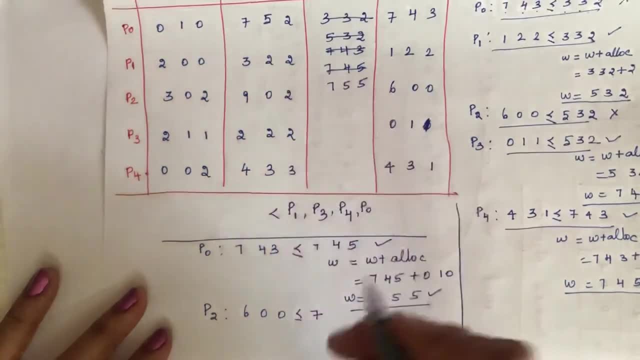 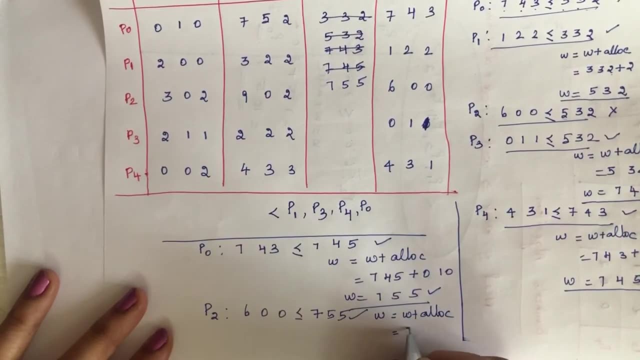 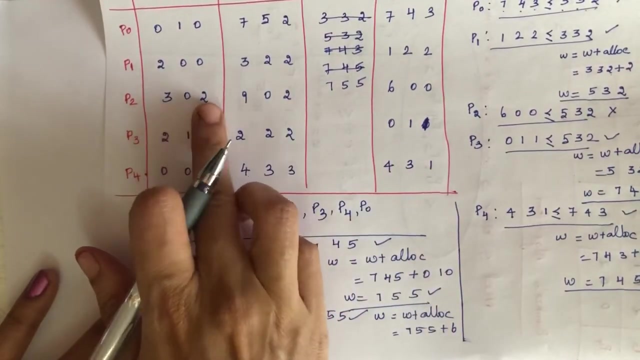 Which is lesser than or equal to 7, 5, 5,. yes, lesser work value will be work plus allocation. Work is 7, 5, 5 plus allocated value for P2 is 6: 0. allocated value for P2 is 3 0, 2 it. 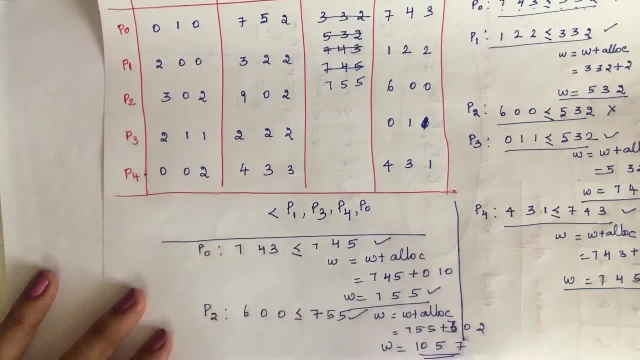 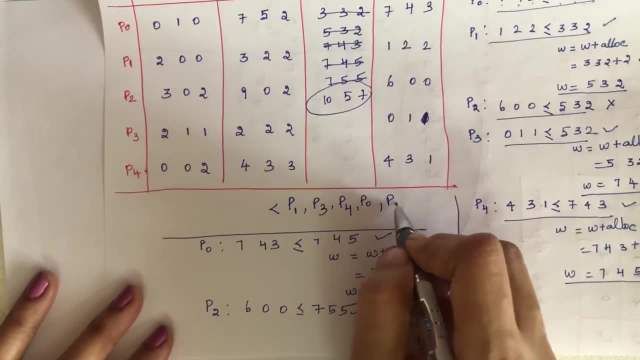 will be 10 5 7. ok, that is the new work value, So we will change this as 10 5 7.. So we will add this P2 to the safe state. So when for the given problem, this is the safe state. 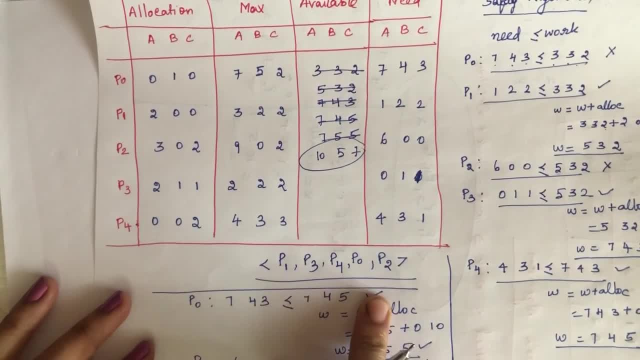 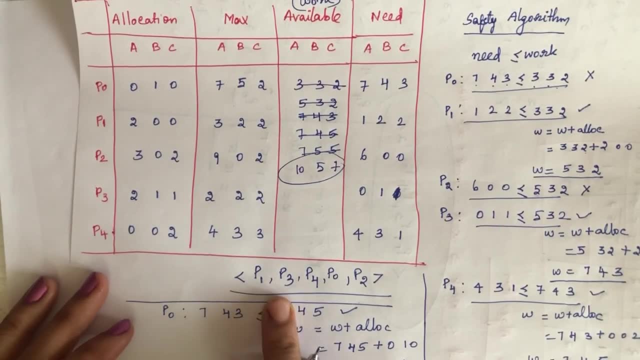 So when the system allocates the resources in this order, it will be in the safe state. It will not go into any deadlock. So in this video we have discussed how to use safety algorithm to find out the safe state. ok, Thank you all for watching.